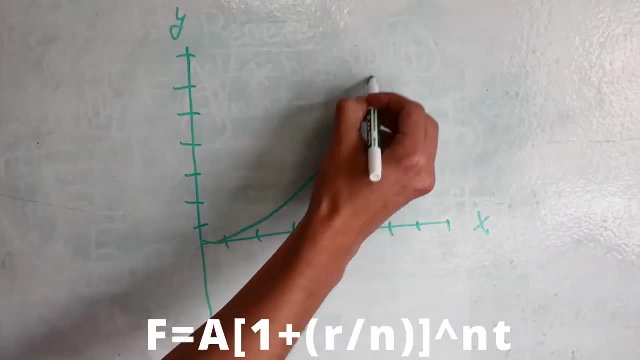 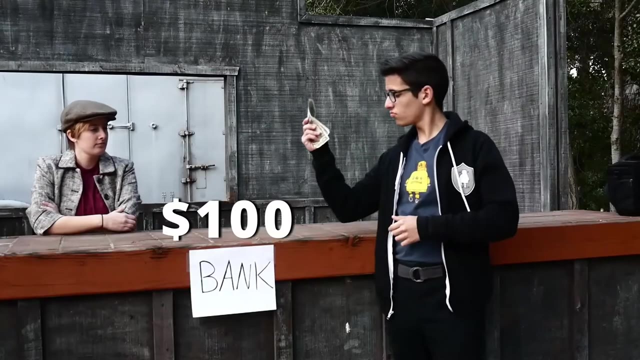 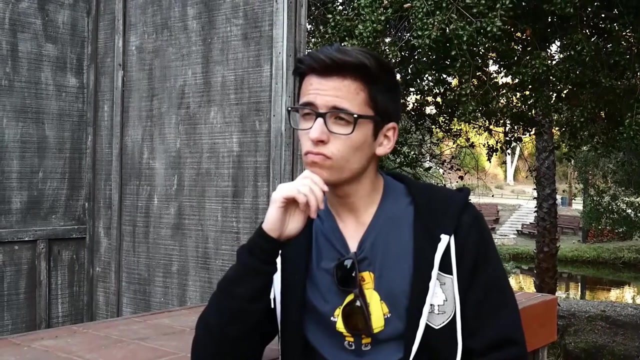 works, There will be an exponential increase in my savings over time. So where do logarithms come in? Let's say I'm an ambitious young man and want my initial $100 to increase to $500 purely off my compound interest of 5%, And I'm just curious how long exactly will? 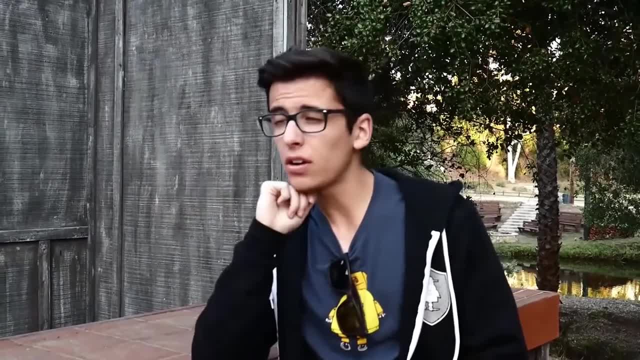 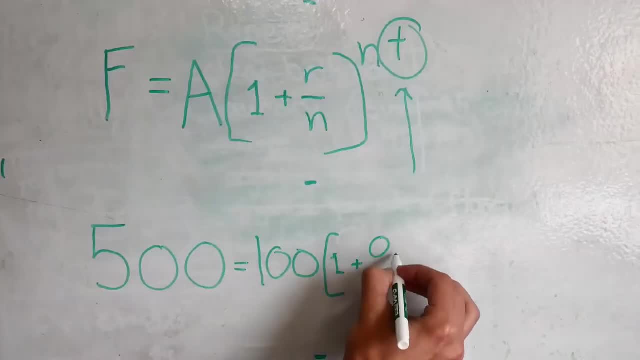 it take me to reach $500 off 5% compound interest. The banker may tell me I don't know, but it's going to be sure heck long of a time, But I still want to know. So now we have a variable t as the exponent, and that's where our problem lies. How will we solve for t? 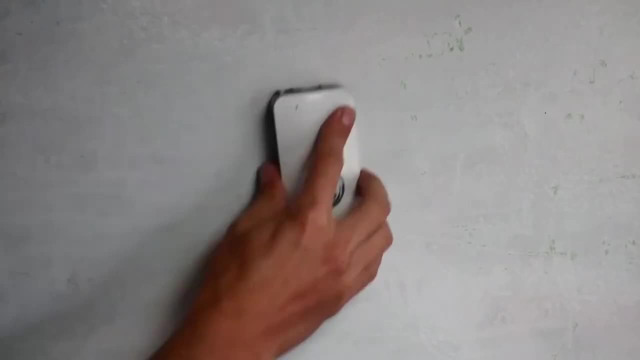 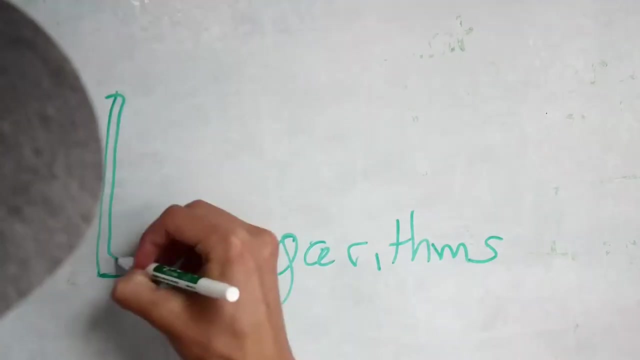 We need to isolate it on one side of the equation and we can't do it with multiplication, addition, division or subtraction, But we can do it with logarithms. Here's how A logarithm is not a complicated concept. For example, the exponential equation 3 to the 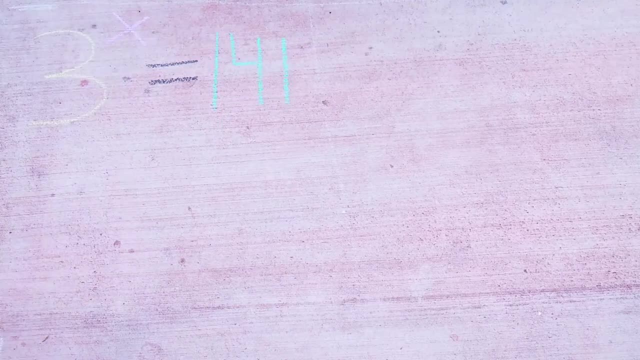 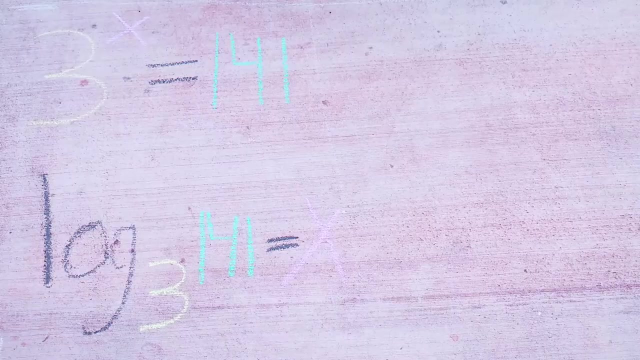 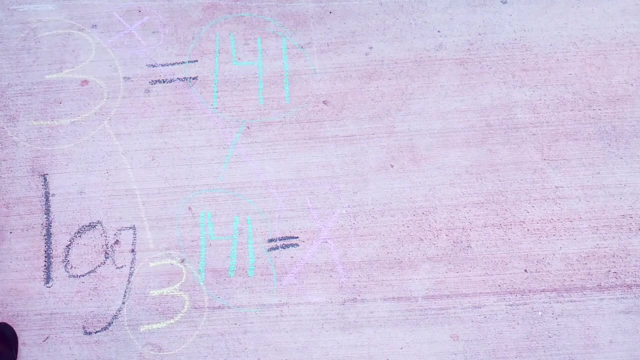 power of x equals 141 is equivalent to the logarithm log base. 3 of 141 equals x. You can observe that this logarithm is simply a rephrasing of the original exponential equation With an important difference: The variable exponent is isolated on one side of the equation. 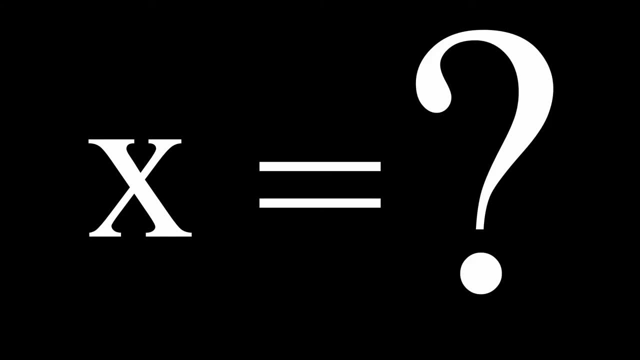 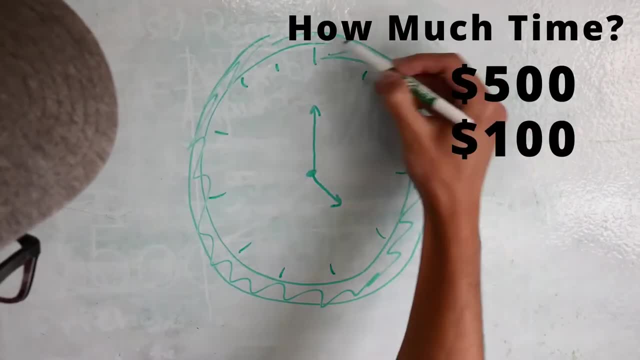 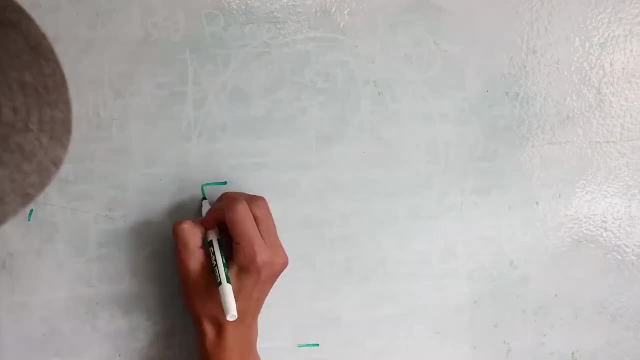 Now we can solve for x. This allows me to answer my compound interest question. How much time will it take me to get $500 from my original $100, compounded monthly at 5%, If we input all of this information into the compound interest equation and simplify it? 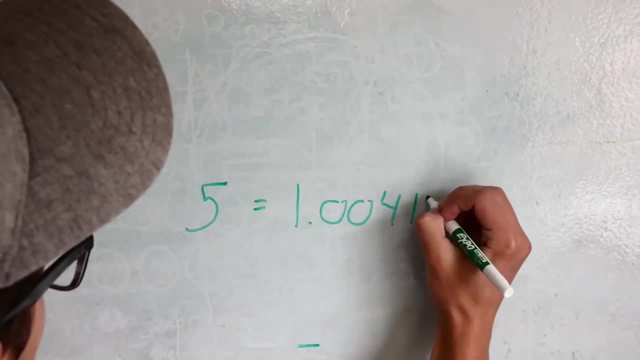 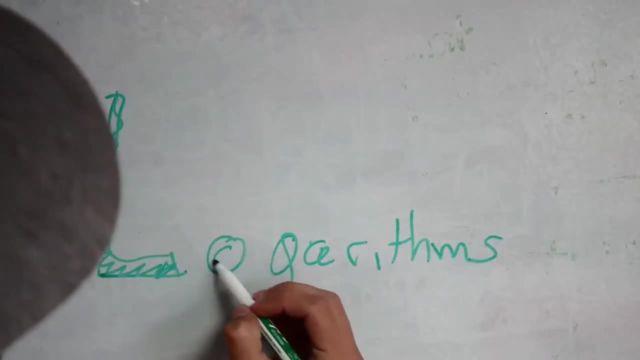 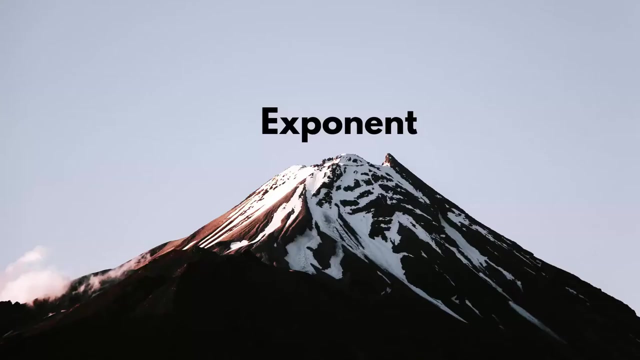 we have 5 equals 1.00417 to the power of 12t. Here's where logarithms come in. In this case, we will be using another rule of logarithms which says that a to the power of x is the same as writing x times. log of a Notice. how? 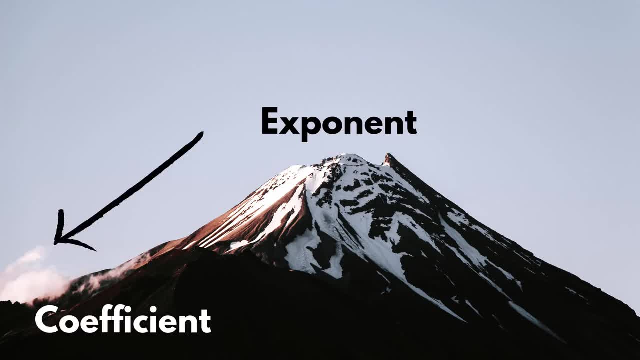 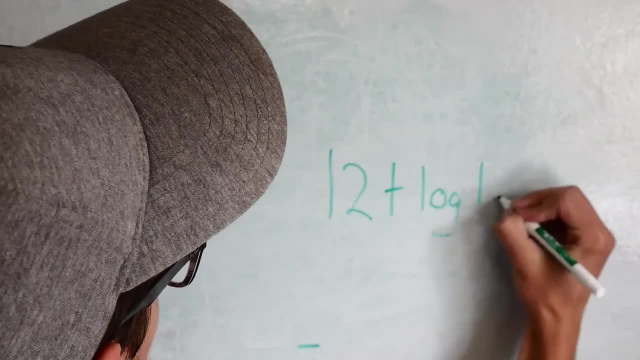 the x is now not an exponent anymore and can be solved as a coefficient. We will use this rule of logarithms on our equation. We can write 12t times log of 1.00417, effectively bringing the variable t down from the exponent to a place it can be easily solved. We can: